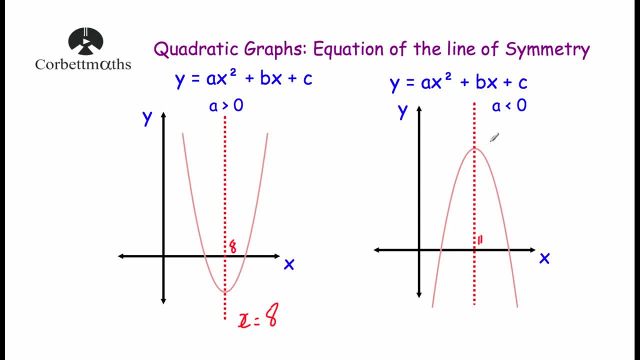 the number 11 on the x axis, the equation of the symmetry would be x equals 8.. And this line of symmetry for this parabola would be x equals 11.. So the line of symmetry of a quadratic graph will be a vertical line and to find the equation of the line of symmetry, 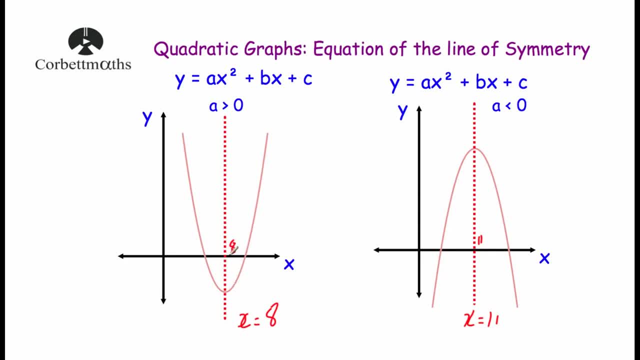 all we need to do is find where the vertical line crosses the x axis, and then it would be: x equals that number, And that's it. Okay, let's have a look at some questions. So here we've been given a quadratic graph. 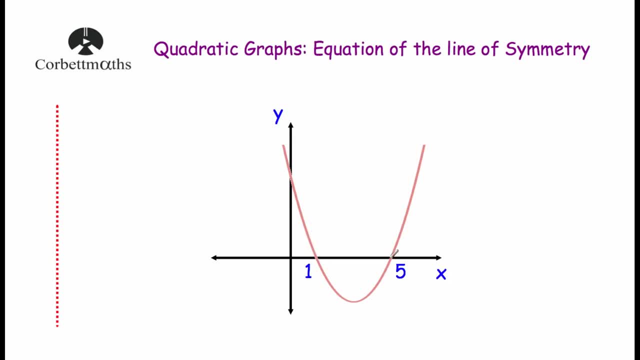 and the quadratic graph crosses the x axis at the point 1 and again at the point 5.. And we've been asked to find the equation of the line of symmetry of this quadratic. So, as you can see, it's symmetrical. so the 1 is the same distance from the mirror line as 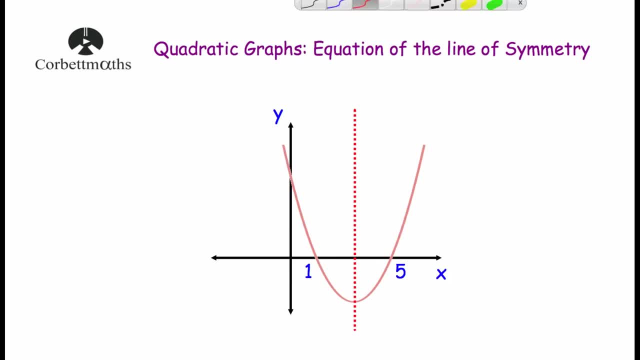 the 5,. so this line will pass through the middle, And because it's passing through the middle, we know it's going to be 3, it's going to cross the x axis at 3.. So that means the equation of this line of symmetry would be: x equals 3.. Now, sometimes, rather than drawing, 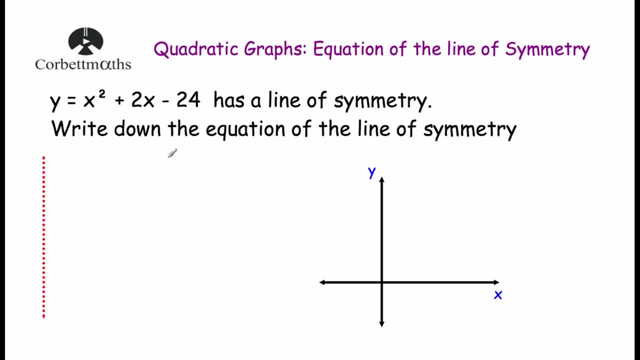 the quadratic for us. we have to figure out what the quadratic looks like ourself. So here we've got a question where we've been given y equals x squared plus 2x minus 24, and it's got a line of symmetry and we've been asked to write down the equation of the. 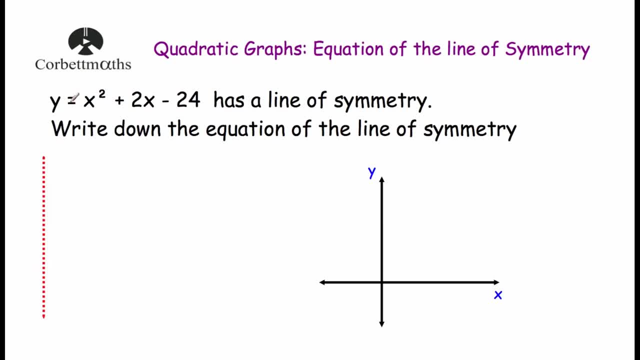 line of symmetry. Now, I've chosen this quadratic on purpose, because what we're going to do is we're going to sketch it and find where it crosses the x axis, and we're going to find our line of symmetry that way. Now there are questions where the graph doesn't actually 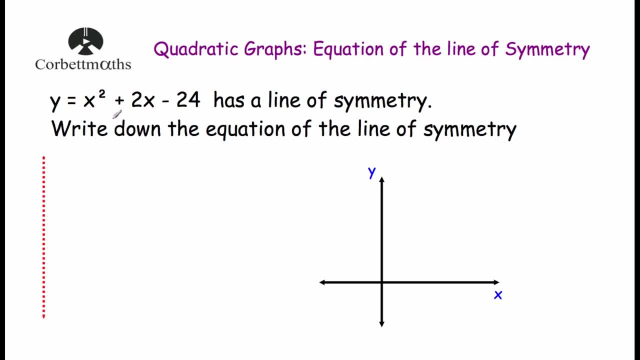 cross the x axis and we have to use a technique called completing the square and no transformations of graphs to do that, and I'll talk a bit about that after this example. So we want to find where this graph crosses the x axis, So to find where a quadratic crosses the x. 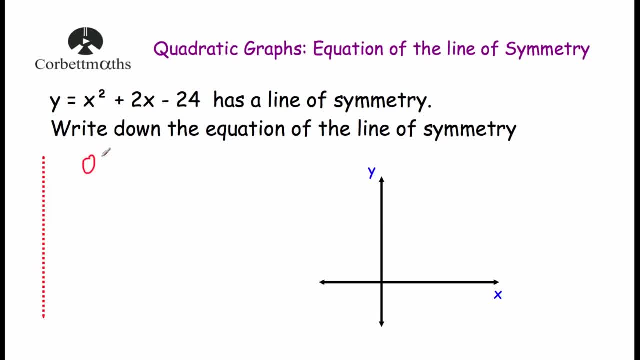 axis, we need to find the x axis. So to find where a quadratic crosses the x axis, we need to find the x axis, so we need to find the. Now, to find where the gradient crosses the x axis, we need one new diagram. So we've been called to a negotiation which is going: 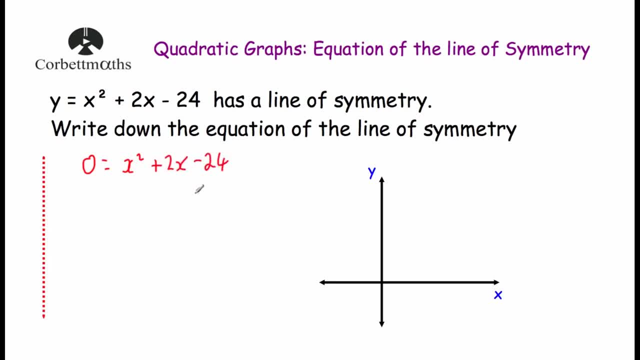 to be one Excellent Egg liver, and what we need is a four령 Now to find where it crosses the x axis. the exotic mommy speaks this equation, So we're going to factorize it, So to put x as the frontier of the brackets, We're going 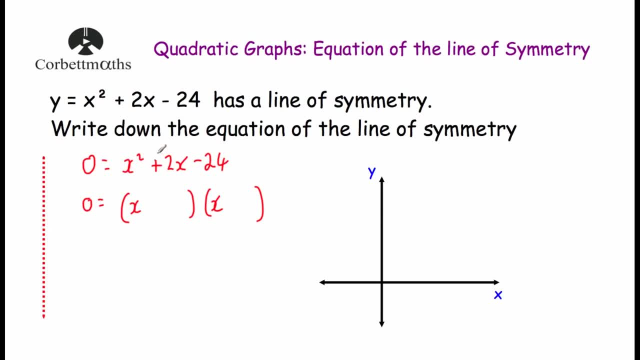 to have two numbers that will multiply together to give us minus 24, and add together to be 2.. So that means because the times are going to be a negative, it means that one of them is a positive and one of them is a negative. We're going to look for numbers that times. 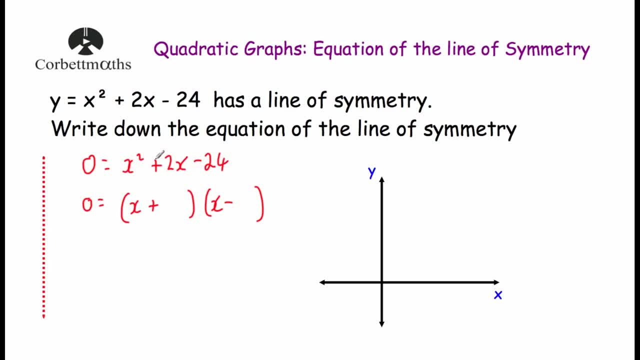 to give to be minus 24.. so I'm thinking 6 and 4, and we want them to add together to be 2, so it's going to be plus 6 and minus 4.. Now to find the values of x. well, we want our brackets to equal 0,. 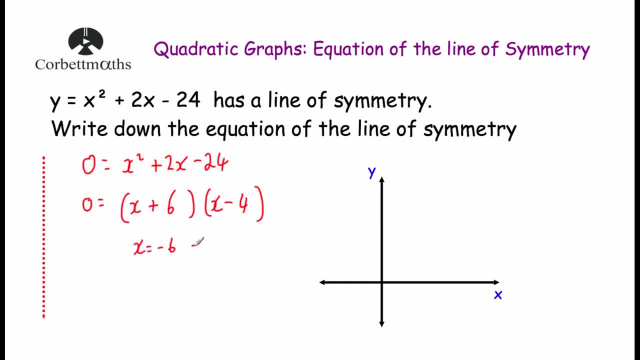 so in this case, x will equal minus 6, and here or x will equal 4.. So that means that our quadratic graph will cross the x-axis at the points minus 6 and 4, so it's going to look something like this: 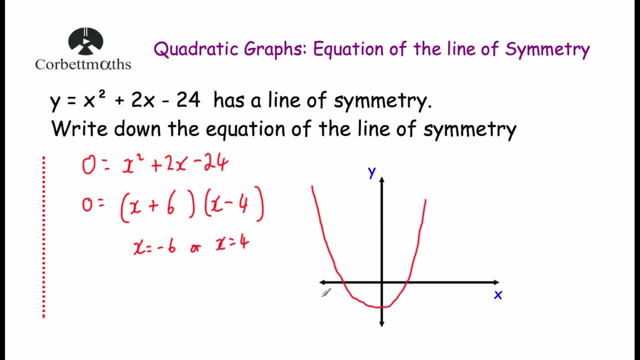 Please excuse my bad sketch. It's like that And it crosses at minus 6 and 4.. Now we know our line of symmetry passes through the middle of our parabola, so it's going to look something like that And we know that it's in the middle. so to find this point, 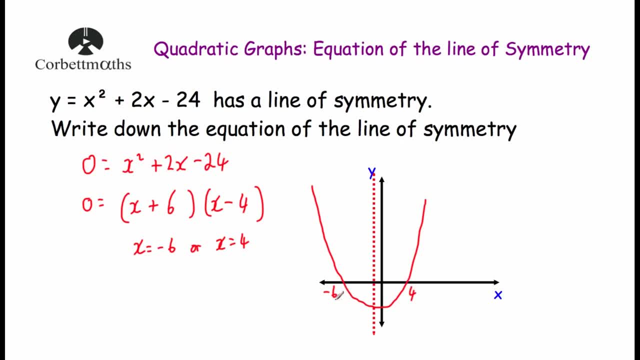 we just need to find the middle of 4 and minus 6.. So we can do that by adding them together and halving it, so we could do minus 6 plus 4, which is equal to minus 2, and minus 2 divided by 2 is equal to minus 1.. 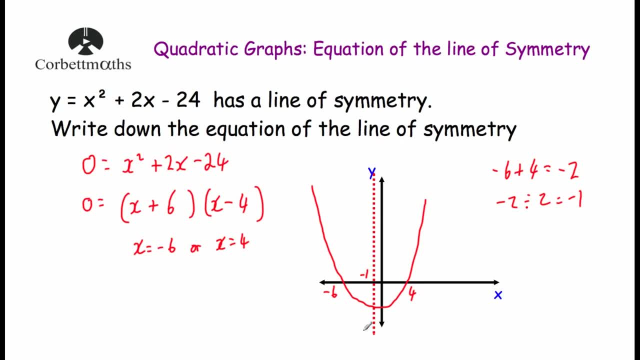 So that means that this mirror line passes through minus 1 on the x-axis. so this equation would be: x equals minus 1.. And that's it, Okay. so we've looked at how to find the parabola, the equation of the line of symmetry for quadratic graphs that have been drawn for us. 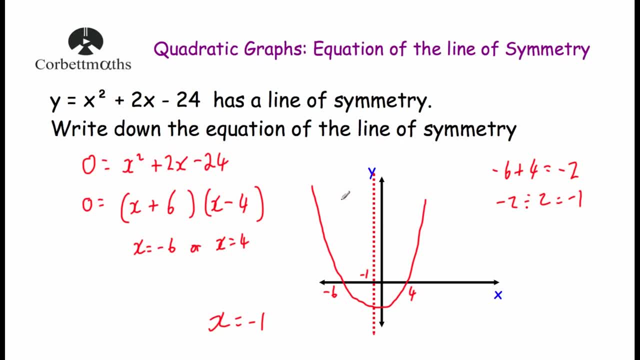 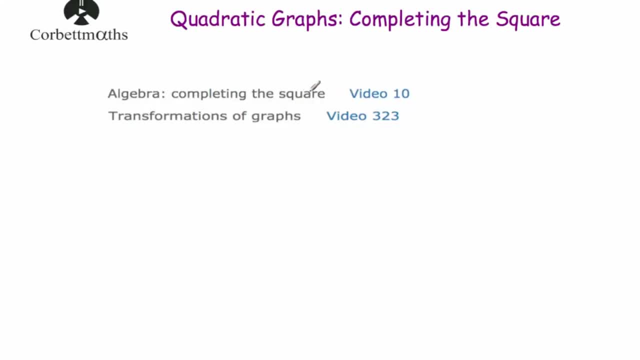 or quadratic graphs that cross the x-axis. Now let's look at a technique which will help us find the equation of the mirror line really easily by using completing the square and transformations of graphs. There's two videos that you would need to watch. before you watch this video, 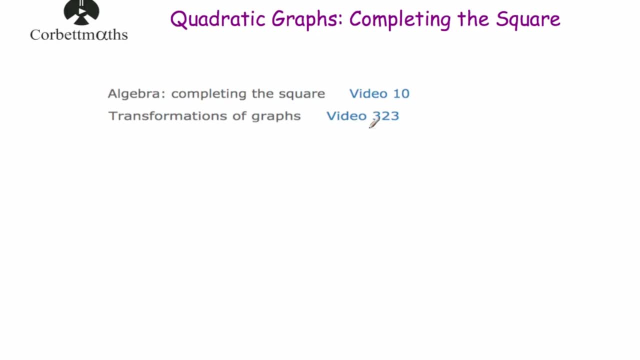 That's video 10 on corporate maths on completing the square, and video 323 on corporate maths on transformations of graphs. I'm going to take it that you know those two topics pretty well throughout this explanation. Here we've got the graph. Y equals x squared. 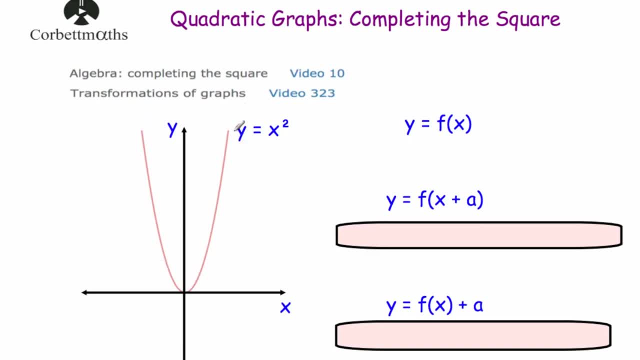 And, as you know, with the graph of y equals x squared. it's a parabola, or you might have called it a u-shaped graph, but it's a parabola and it goes through the point 0,, 0, or the origin. 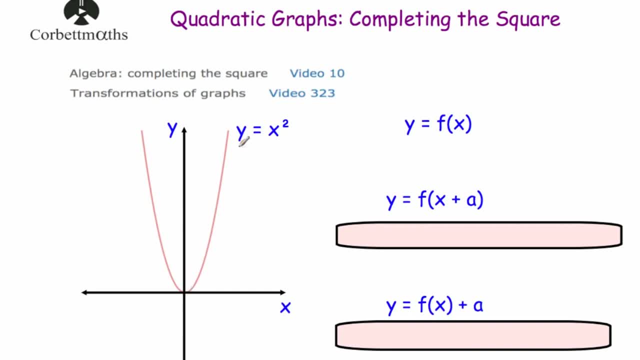 because obviously 0 squared is 0.. So that's the graph: y equals x squared. Now, if you've watched the transformations of graphs video, you'll know that if you consider, if you let that equal y equals f of x, that x squared graph. 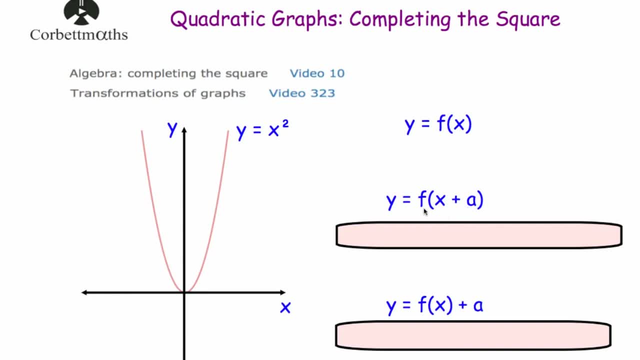 if you add a number to that x inside of the brackets, it will move the graph a squared to the left. Okay, So in other words, if this graph here is y equals f of x, the graph of y equals f of bracket x plus 2. 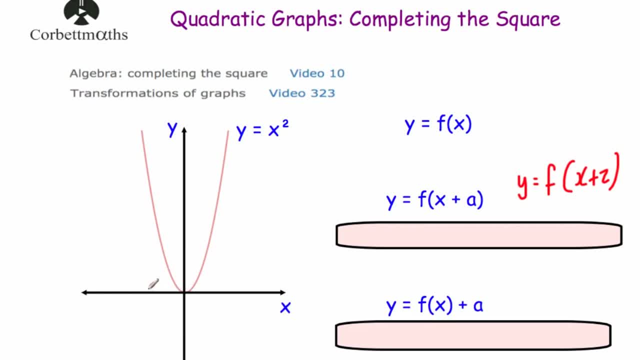 would be the same graph but shifted, or translated, two squares to the left. So instead of having a turning point at the origin, it would have a turning point at the point minus 2, 0.. So that's going to be very useful in this topic. 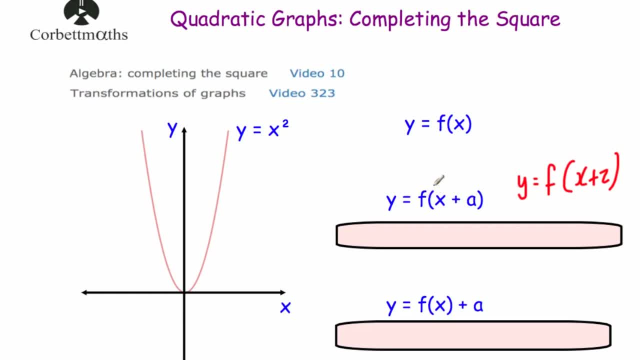 If it was a minus. so if it was: y equals f bracket, x minus a. it moves through, translates the graph: a squared to the right. it's sort of counterintuitive. I always say to my students: Next, what we're going to do is we're also going to consider 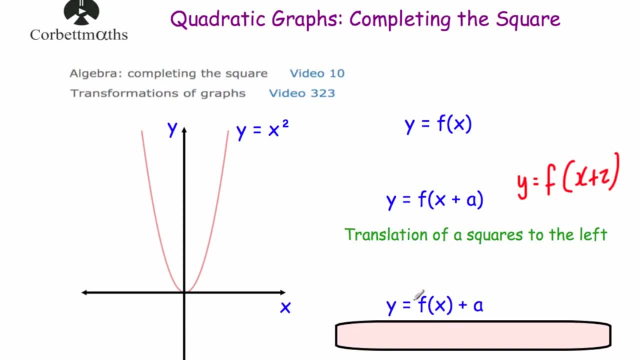 what happens when you add outside of the brackets, In other words, y equals f of x plus a, over the a's outside of the brackets, that moves the graph or translates the graph a squares upwards. So if it was, y equals f of x plus 3,. 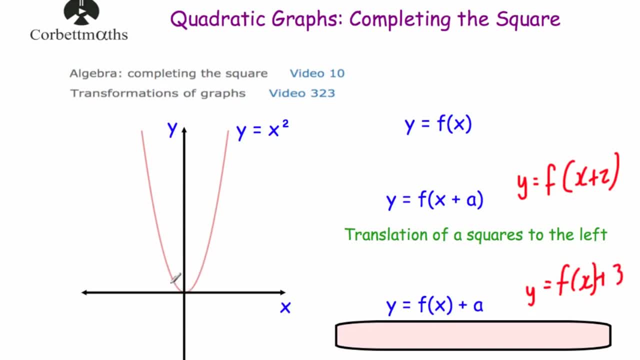 it would move the graph three squares upwards. So instead of it having a turning point at the origin, the graph would have a turning point at the coordinate 0, 3.. So those two transformations are very important for this topic. They're going to be very helpful for this topic. 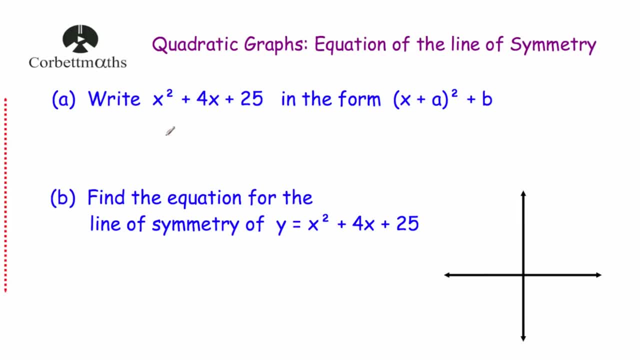 Okay, so let's have a look at our first question using completing the square to find that equation of the line of symmetry. So part a says: write x squared plus 4x plus 25, in the form x plus a close bracket, squared plus b. 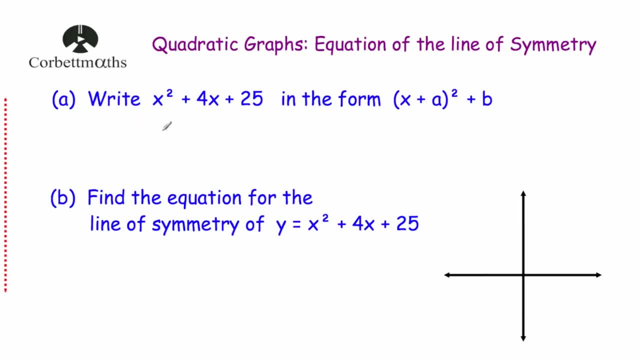 So, in other words, we're going to do completing the square on this expression. So we're going to open our brackets and write x plus- now we always have this coefficient of x- and put it in the brackets. So half of 4 is 2,. 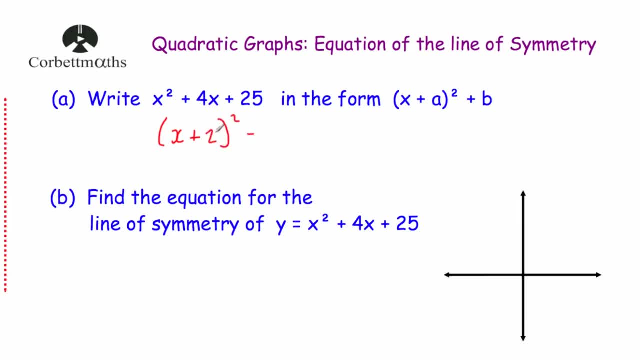 close bracket squared and then we subtract whatever this number is squared. so 2 squared is 4. so we're going to subtract 4 and then put our plus 25 on the end and then, whenever we simplify this, we will get x plus 2, close brackets squared and then minus 4 plus 25 is plus 21. so x squared plus 4x plus 25. 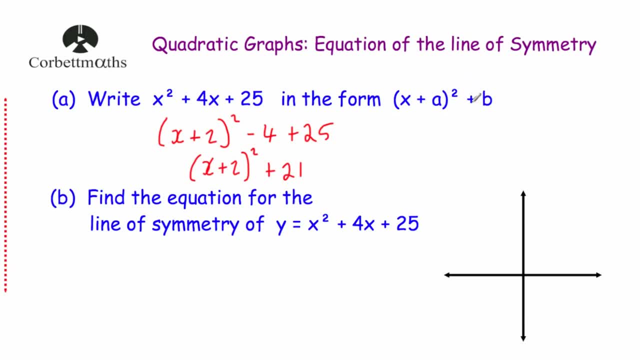 in the form: x plus a, close brackets, squared plus b, is equal to x plus 2, close brackets, squared plus 21, and you can check that expanding this would give you x squared plus 4x plus 4, and then plus 21 would give you your plus 25. so part b says: find the equation of the line of symmetry of y equals. 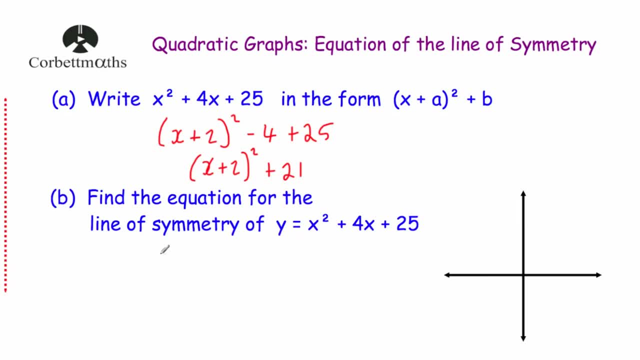 x squared plus 4x plus 25. well squared, because we've done completing the square on it. so we've got x plus 2- close brackets- squared plus 21. now let's start off with our x squared graph at that u-shaped parabola. now, considering transformations of graphs, we know that this plus 2 will move the. 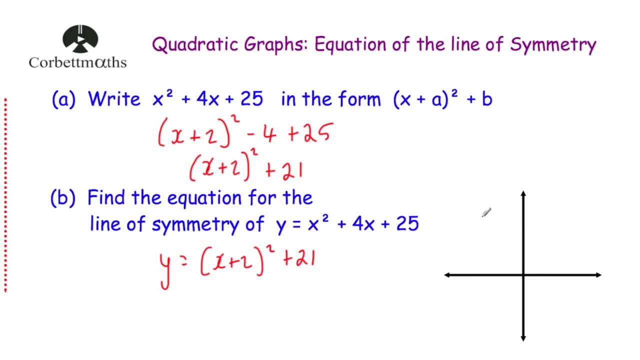 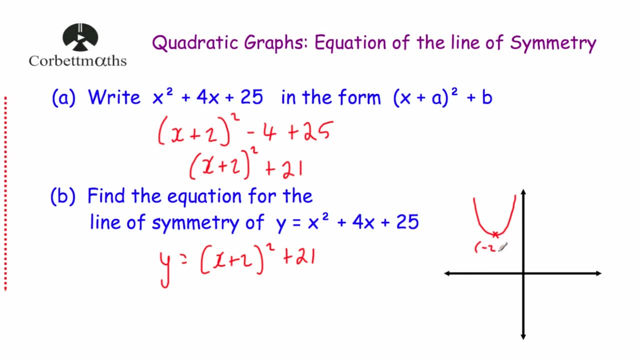 graph two squares to the left. so x squared graph will move two squares to the left and look something like that, and then the plus 21 will move it up 21. so our parabola would look something like that. so that point that was at the origin will now be here, which was: it's been moved two to the left, so that's minus two and 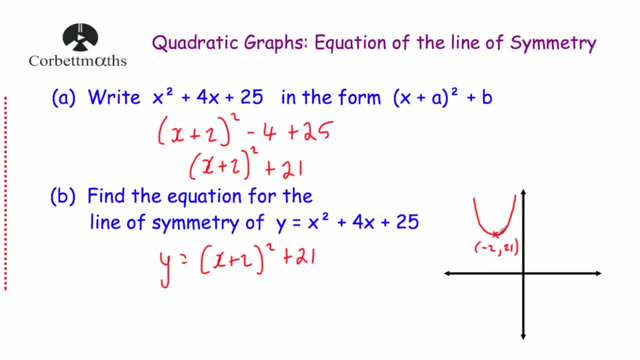 then move 21 up, so it's 21. so the coordinates at that point will be minus 2, 21. now we want to find the equation of the line of symmetry of this parabola. so we consider that line of symmetry. it'll go straight through that minimum point and through the x-axis and that line of symmetry. 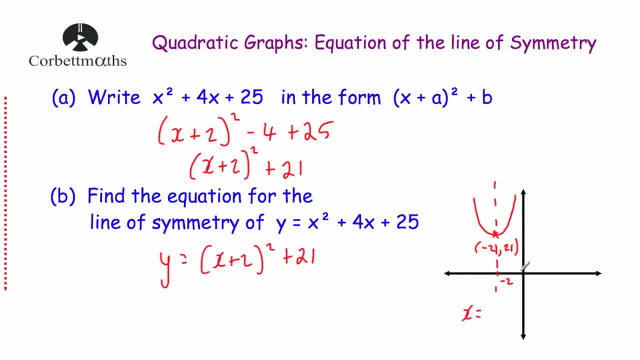 would be x equals, and it'll cross the x-axis at minus 2 because it's moved two to the left. so it'll be x equals minus 2, and that's it. so the equation of the line of symmetry of y equals x squared plus 4x plus 25 would be x equals minus 2, right? so let's have a look at one last example. 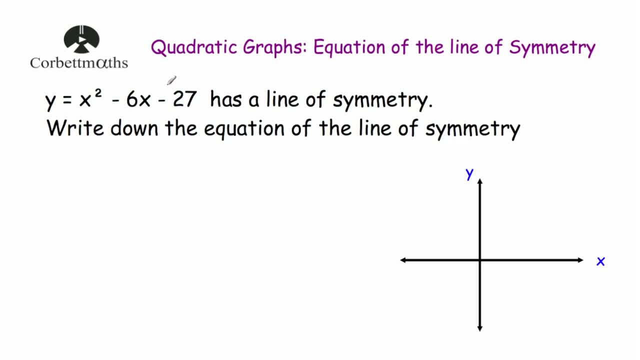 so we've got y equals x squared minus 6x minus 27, and we've been told it's got a line of symmetry and we've been asked to find the equation of that line of symmetry. so let's start by N수 squared x squared minus 2y squared plus 5y. squared minus 2y squared minus 2y squared minus. 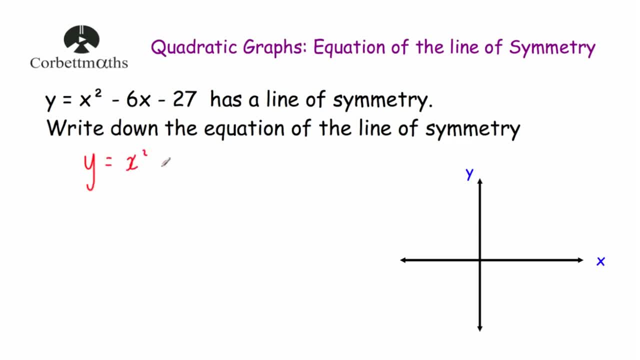 writing down the equation off the quadratic y equals x squared minus 6x minus 27, and we're going to do completing the square on this. so we're going to write: y equals, then brackets x. now half of minus 6 is minus 3, so minus 3, close, brackets squared. then we subtract whatever this. 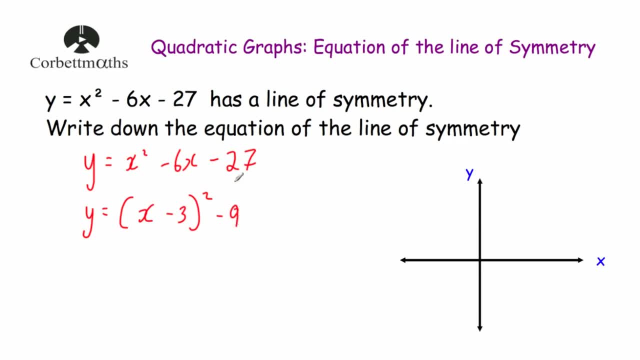 is squared. well, minus 3 squared is 9. so subtract 9 and then we put our takeaway 27 on the end. so minus 27. so simplifying this will give us y equals open brackets, x minus 3 squared, and then minus 9. takeaway 27 will be minus 36. so we've done completing the square on our quadratic. now we can.